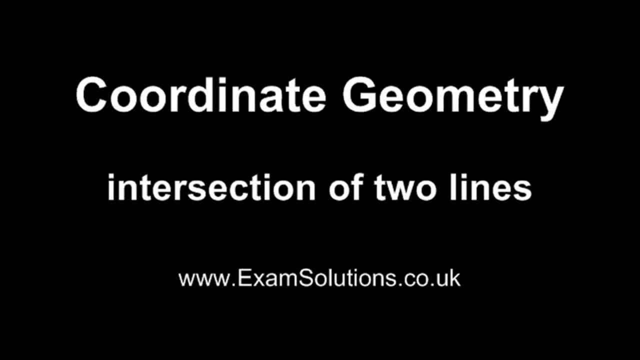 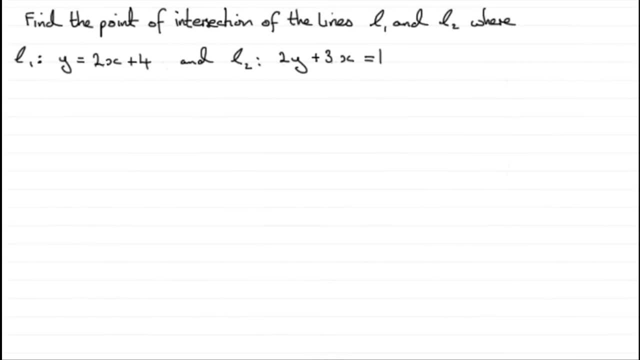 Hi, welcome to this tutorial on finding the intersection of two lines. Now, the best way I can think of illustrating this is by way of an example, And what we've got here is find the point of intersection of the lines L1 and L2, where L1 is such that y equals. 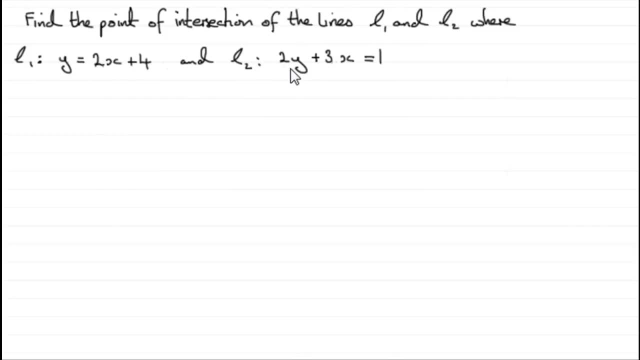 2x plus 4 and L2 is such that 2y plus 3x equals 1.. Now, before we start, what I would always encourage you to do is draw a sketch, And the reason for that is because if you draw a sketch, you've got every chance of recognising if your answer looks sensible. 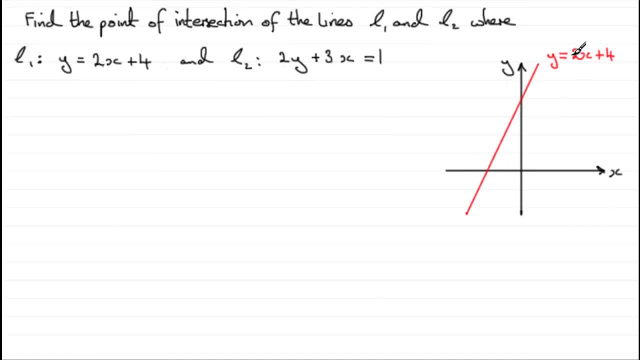 So to draw the sketch then of say y equals 2x plus 4, we know it's going to be a straight line And it's in the form: y equals mx plus c. So we know that it crosses the y axis when x is 0, making y 4.. So we can write this point in here as 4.. Let's just mark that in there. 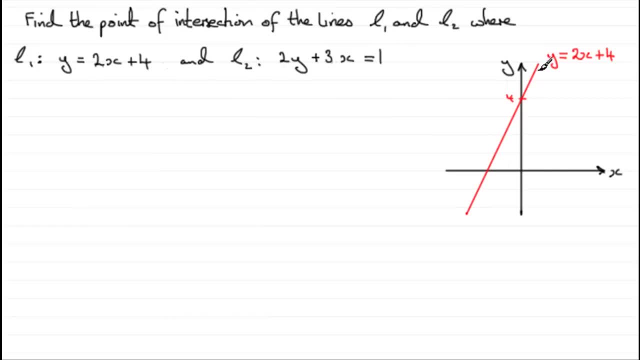 It's got a gradient of 2, so it's going to slope upwards, And so it's going to look something like this. You might even want to find this point where it crosses the x axis, That's when y is 0. And that would mean that x was 0.. 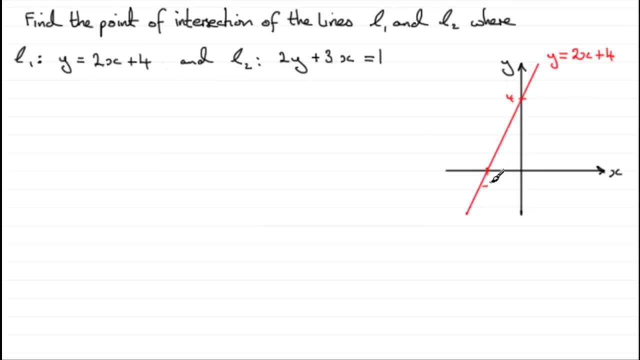 Minus 2.. So that's quite useful to have that point in there. And for line L2, well, we could rearrange it similarly in the form y equals mx plus c and sketch it from there, Or we could just find out where it crosses the x and y axis. 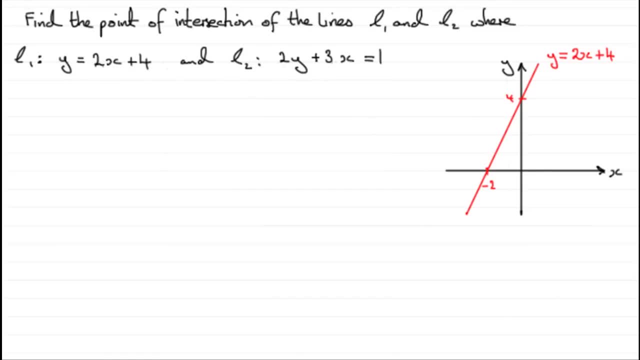 by putting x and y individually equal to 0.. Whatever system we use, we'd get something like this: OK, Now, that means that this point is where the two lines intersect, And you can see that. OK, Now, that means that this point is where the two lines intersect, And you can see that. 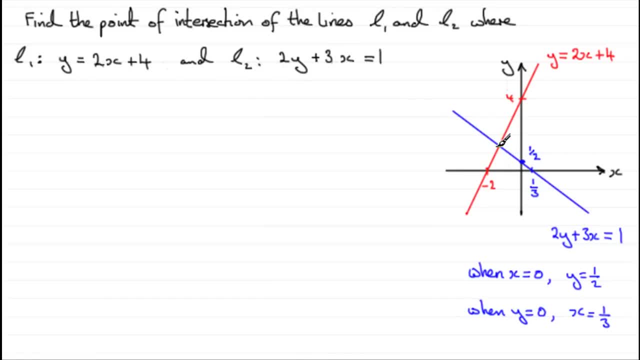 OK, Now, that means that this point is where the two lines intersect, And you can see that that this point will have an x coordinate something greater than minus 2.. And its y coordinate will be less than 4.. So that gives us some idea, then, what to expect. 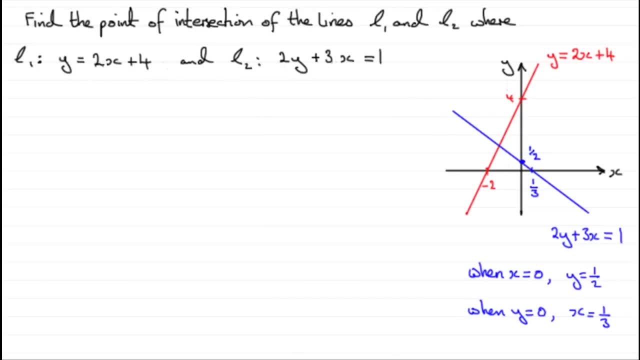 OK. Well, how do we find this point of intersection? Let's label it. Let's say we call it A. So if we were trying to find that point A, let's give it a subtitle here for A. what we need to do is solve our two equations simultaneously. That's because at this point we're looking. 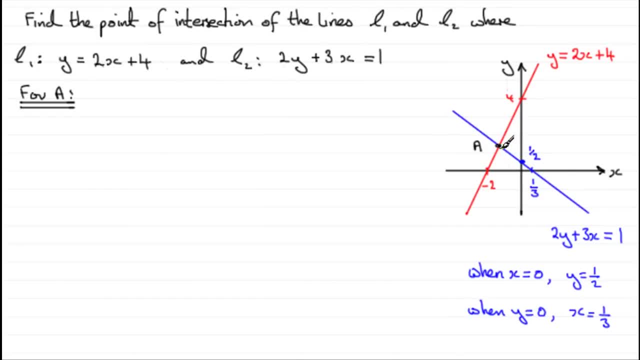 for a value of x and y that not only satisfies the blue line, but also satisfies the red line. It satisfies both these equations, And that's what simultaneous equations is all about. So to solve these two simultaneous equations, I would write each of them out. OK, So we've. 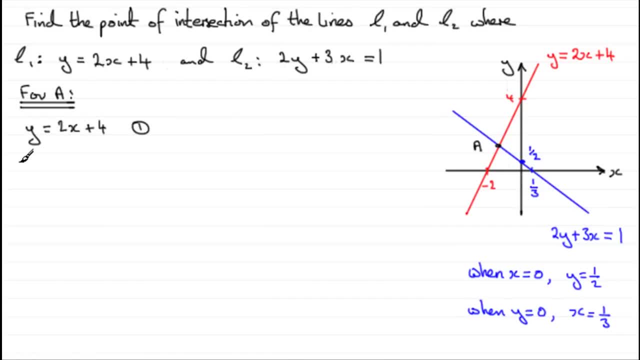 got: y equals 2x plus a. So we know the following: We know that x is equal to a, So let's give plus 4 and number it in the usual way, and we've got the other one. 2y plus 3x equals 1.. Now for 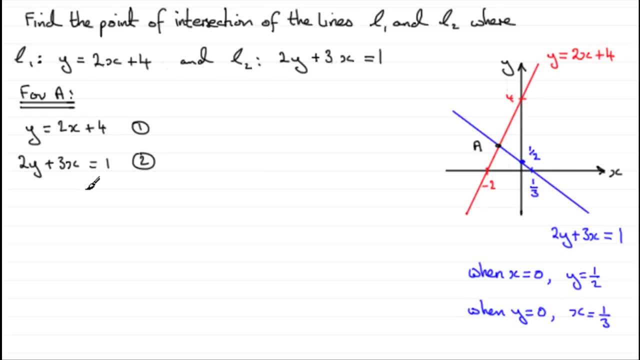 something like this: two linear equations. I could do it by the method of elimination or by substitution. I'll do the elimination at the end because for this example it seems to work better for substitution, because, look, we've got y equals 2x plus 4y in terms of x. so I could immediately 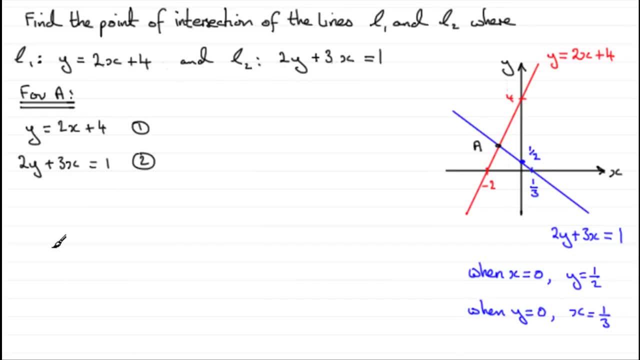 substitute this into equation 2.. So if I do that- let's just put a note here- sub 1 into 2, then we're going to therefore have 2 times whatever y is, which is 2x plus 4, 2x plus 4, and then 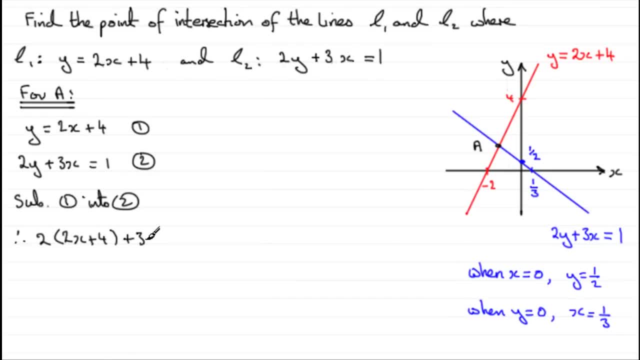 we're going to have 2 times whatever y is, which is 2x plus 4, We've got plus the 3x and it equals that 1.. So we just need to expand the bracket, so we've got 4x plus 8, and then the plus 3x equals 1.. 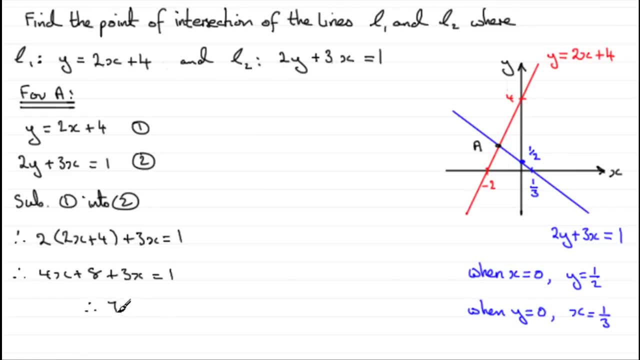 Group together the x's, so we end up with 7x and subtract 8 from both sides, so 1 take away 8 is minus 7.. And if we divide both sides by 7, we end up with x equaling minus 7 divided by 7, which is minus 1.. 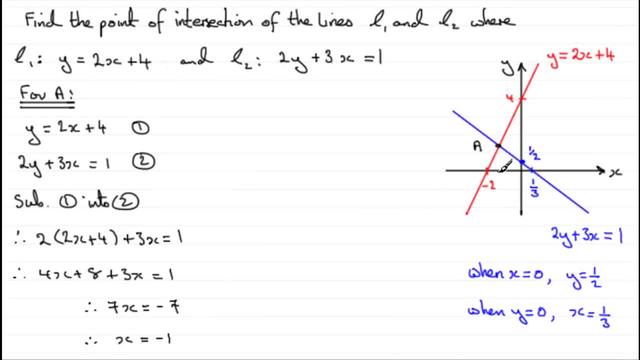 And that's looking quite encouraging because you can see our x coordinate has got to be between 0 here and minus 2, so minus 1 looks pretty good. We need to get that y coordinate, so all we need to do is substitute. let's just write substitute x equals minus 1 into 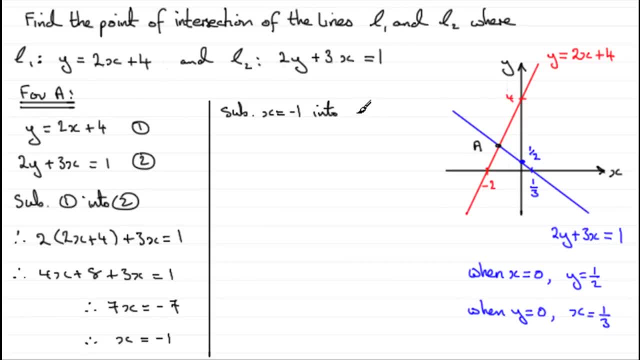 either equation 1 or 2, it would seem sensible to put it into 1, because it gives us y directly. So therefore we have y equals 2 times x, but x is minus 1, and then plus that 4, so we end up with y equaling minus 2 plus 4, which is 2.. 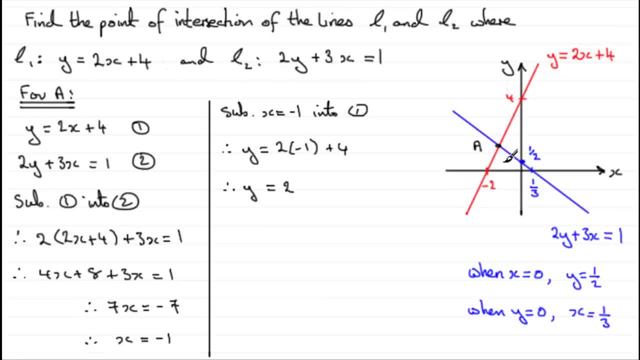 And again that looks sensible, It's got to be more than that half. So in summary, we can just say that therefore, the point of the intersection okay, has to be minus 1, and then the y coordinate is 2, minus 1,, 2, and there's our answer. 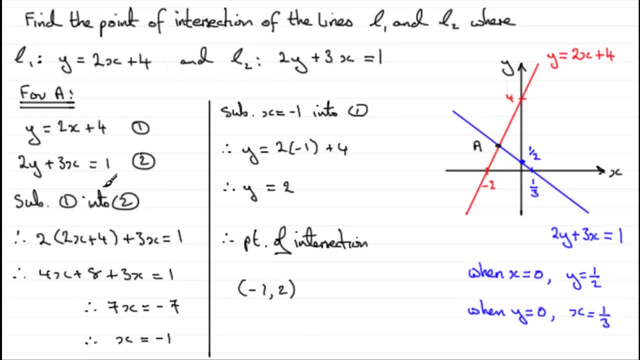 Now, I did say that you could solve these equations by elimination, and I will do that for you now. So if I'm doing this, then by the process of elimination I would want to rearrange equation 1, and also double it. 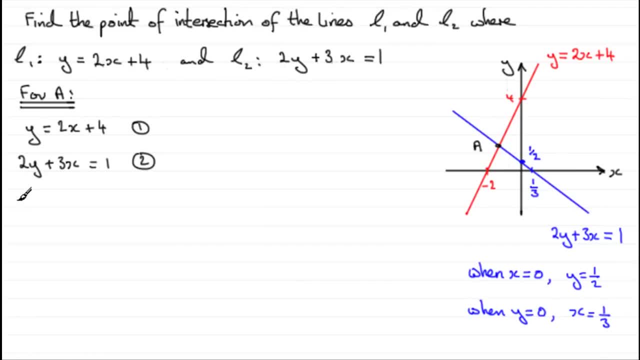 So if I was to double the y, let's say we take equation 1, and we multiply it by 2, and rearrange it, we're going to have 2y. this would be 4x plus 8, but I'm going to subtract that 4x now from both sides. 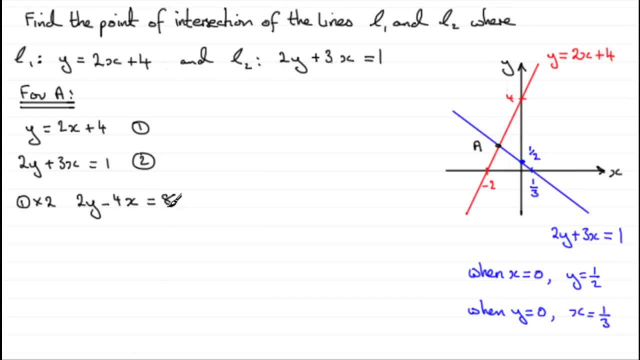 so we'd have 2y minus 4x equals 8, and I would call that equation 3.. We've got equation 2, let's just put it underneath here 2 times 1, if you like. it's going to leave it unchanged. 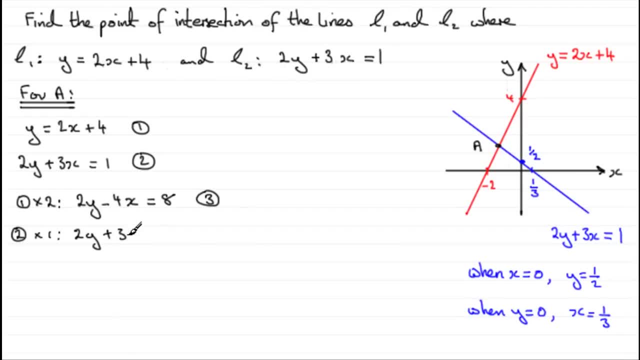 which would just be 2y plus 3x equals 1, and we'll keep that then as 2.. So I can eliminate the y's here by simply subtracting the two equations I'm going to do, equation 3 minus equation 2..